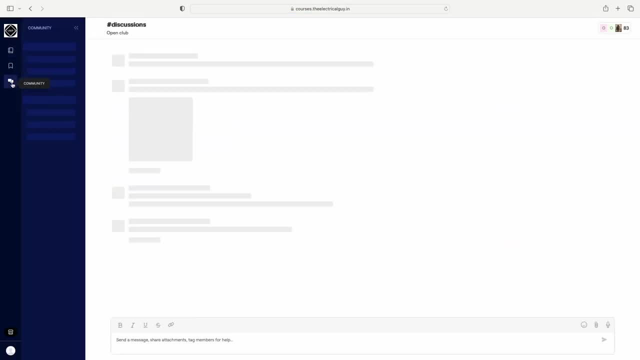 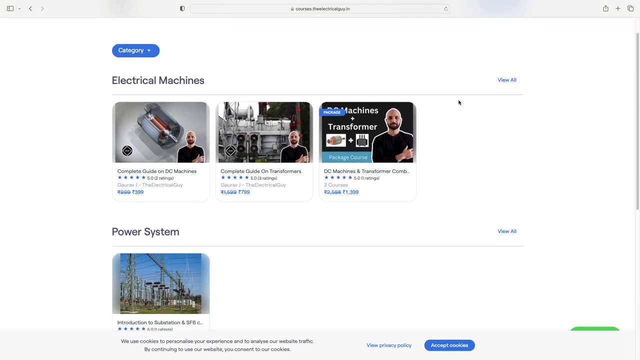 are missing on a lot of things. You are missing on the community features for electrical engineering. you are missing on the easiest courses that i'm offering on the electrical machine and also some of the most popular courses that i'm offering on the electrical machine and also some of the 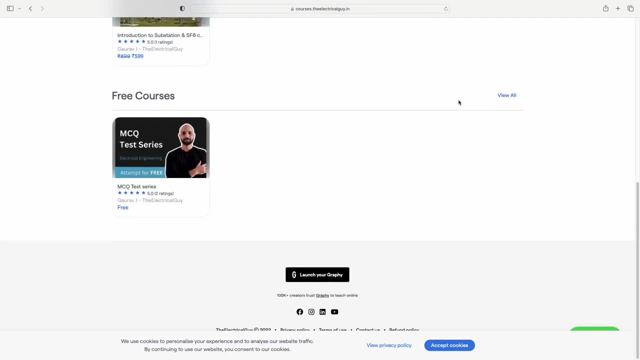 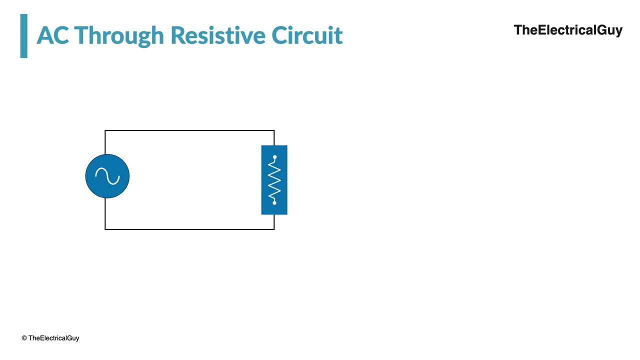 most popular courses that i'm offering on the electrical machine and also some of the most introductory courses on power system. So definitely go and check out login and you will see a lot of good things there. Now let us talk about AC through resistive circuit. 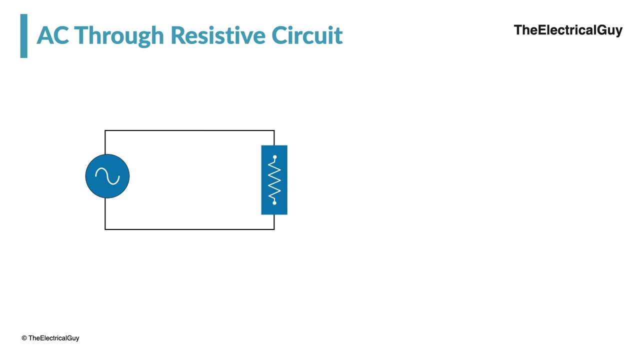 Now we know about the resistance right. resistance simply opposes the flow of electrons. Now it really doesn't matter what is the magnitude of current, whether it's 5 ampere, 15 ampere or 500 ampere, it really doesn't matter. It also doesn't matter that whether the current 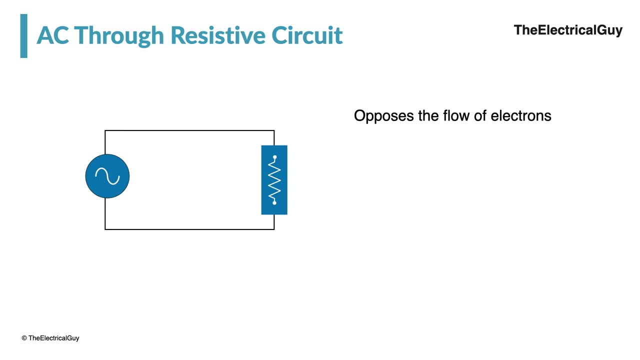 is alternating in nature or is it constant? So anything you that you will pass through the resistor, it is simply going to oppose that flow of electrons, right, and that is the reason why resistor always follows the ohm's law. Now what ohm's law tells us? ohm's law says voltage is. 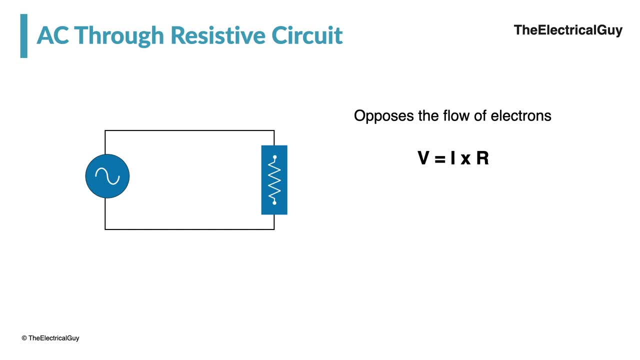 directly proportional to the current, provided the resistance is constant. So if your resistance is constant, then it is pretty much clear that the voltage is directly proportional to the current, and that means when current increases, the voltage will also increase, and similarly, if current decreases, the voltage will also decrease. This is really. 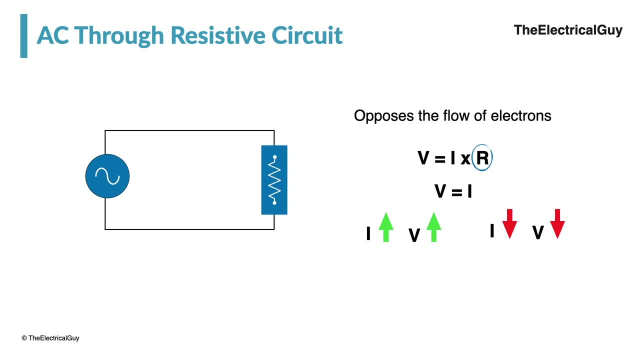 the easiest thing in case of resistive circuit. Now, with the help of this explanation, we can plot the waveforms for current and voltage in case of resistive circuit. So let us do that here Now. first let us plot the voltage. So this is the alternating current waveform, So this is how the current will flow in case of. 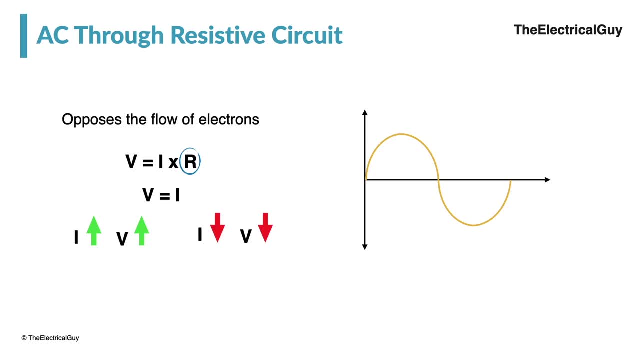 resistive circuit. that is the alternating in nature. Now it is pretty much clear from the explanation that we just saw that when current increases, the voltage will increase. That means when current is maximum, the voltage will also be maximum, and that is the reason why, if you draw the 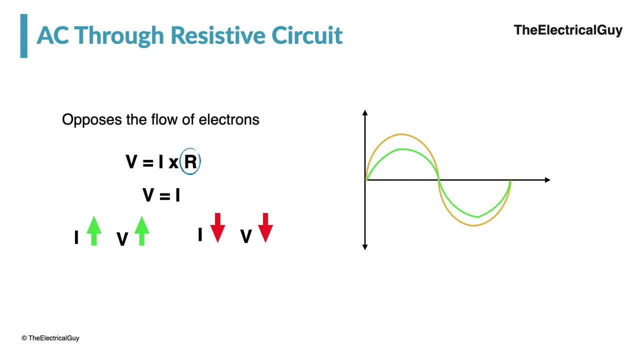 voltage waveform. it will look like this, And from this waveform it is pretty much clear that when current is maximum, the voltage is also maximum. When current is zero, the voltage is also zero. and when current reaches the negative peak, voltage follows, that voltage at the same times becomes the 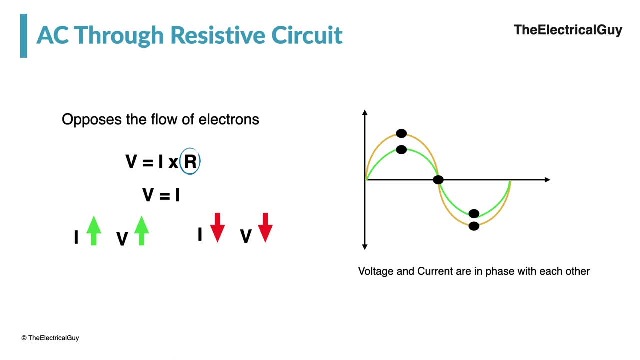 reaches to the negative peak and we can say that voltage and current are perfectly in phase with each other. Right, very clear: when current increases, voltage also increases because of the ohm's law, And similarly, when voltage decrease, current decreases, the voltage will also decrease across the resistor, and hence voltage and current are perfectly in phase with each other. in case of 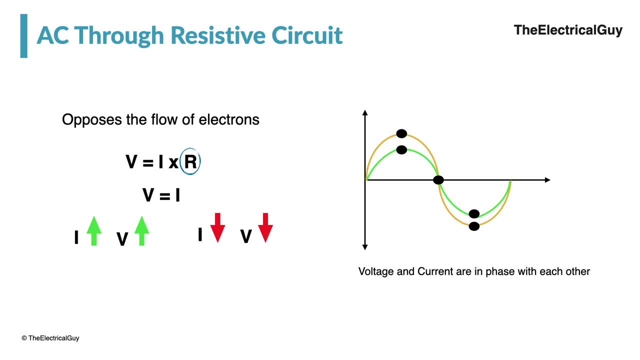 resistive circuit. Right, that is how the voltage and current behave. Now let us understand about the power through resistive circuit. Now, before we understand that, we need to understand one important concept and that is instantaneous power. Say, for example, I want to calculate the power at this particular instance where 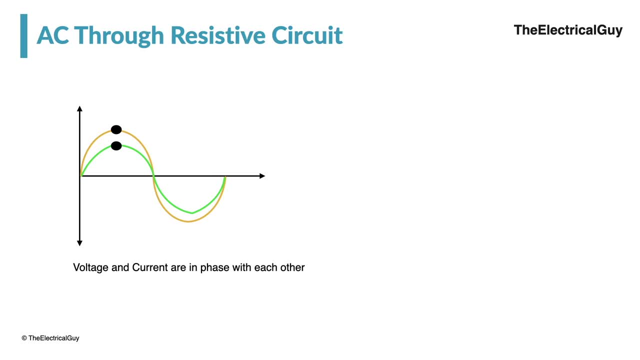 voltage and current. both are maximum. Now, to calculate the instantaneous power at this particular instance, what I have to do is I have to simply multiply the current max times the voltage max, and that will give me p max. Now, this power that we will be getting from this is only true. 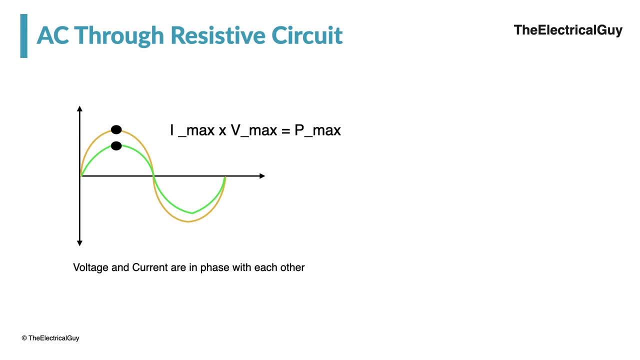 for this particular instance, where voltage and current both are maximum, and this power will not be true for any other instance on the waveform, And hence this power is called as instantaneous power, because we are measuring the power at a particular instance and hence it is called as. 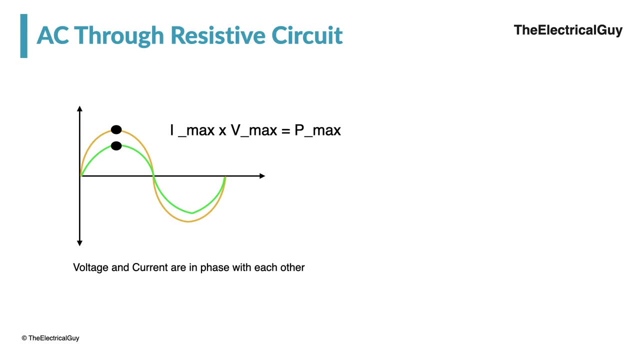 instantaneous power. Now, in case of resistive circuit, where voltage and current are perfectly in phase with each other, you calculate instantaneous power at any given instance and you will always get a positive power. So let's say, even if you are, you know, calculating power, when voltage and current are in the positive side, you will get. 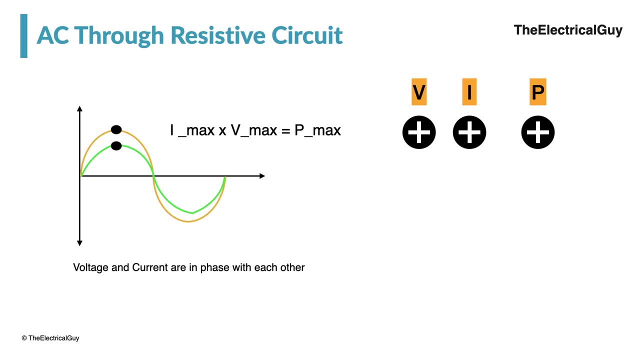 a power as positive. So positive multiplied by positive will give us a positive result. When voltage and current are zero, the power will also be zero. Yes, it, it gets to the zero, but it never gets to the negative side. It will drop to zero, but it will never go to the negative side. 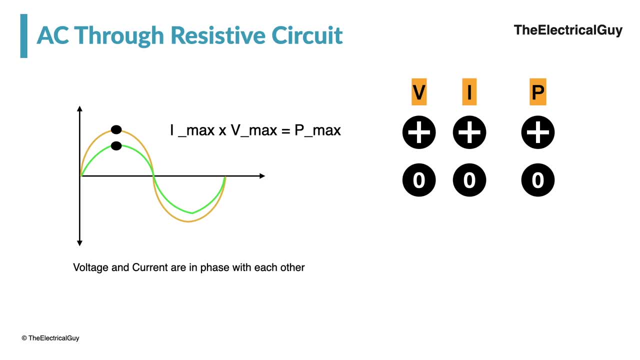 And similarly, when, even when- voltage and current act is negative, you will get a positive output, because negative multiplied by negative gives us a positive output. so you take any instance on this waveform and you will get only positive power. and if you draw the waveform for this positive power, it will look like: 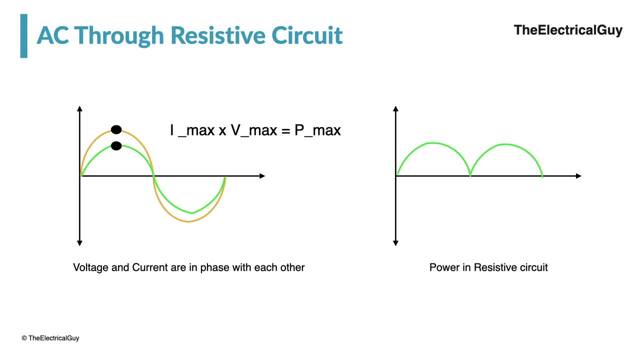 this, and this is the most important property of a resistive circuit: that the power never goes to the negative side. It will always be, uh, on the positive sideı. Yes, it drops to the zero 0, but again it get backs to the positive 0, then positive again, but never to the negative. 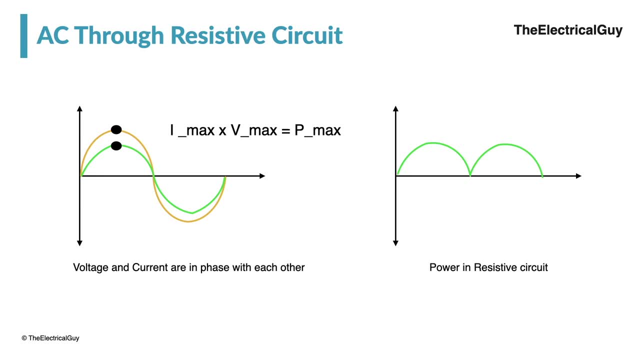 side, and this power is also known as active power. so the power that remains always on the positive side is what we call as active power, and if you are interested in understanding more about active, reactive and apparent power, then I have a dedicated and a very easy to. 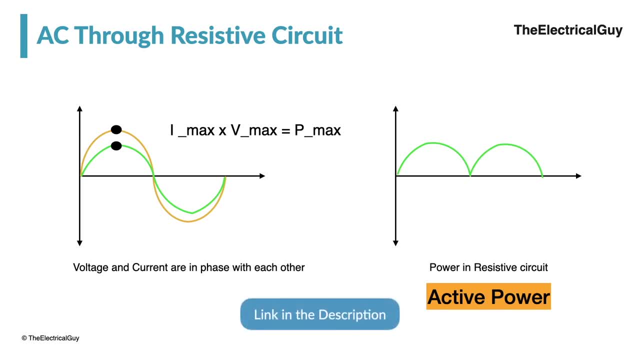 understand video on that. I will give link for that video down in the description. you can check that out. clear. so that's how the power in case of resistive circuit. Now there are two important things that you should remember in case of AC through resistive. 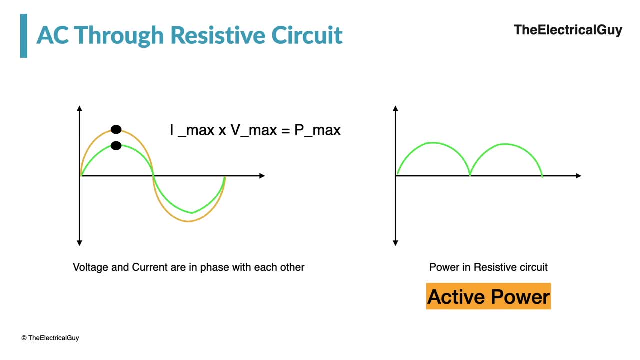 circuit one. in case of resistive circuit, voltage and current are perfectly in phase with each other. Now, what does in phase mean? In phase means voltage and current reaches their positive peak at the same time, they become zero at the same time and they become negative or they reach their negative peak. 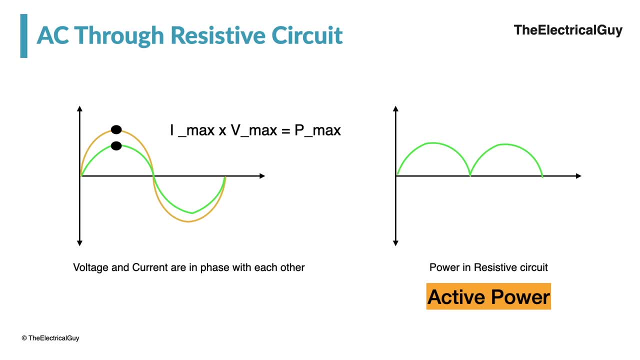 at the same time. So, So, So, So, So, So So that is one. The second point that we need to remember is, in case of AC through resistive circuit, the power always remains positive. It never goes to the negative side, Right? So I hope you understood something useful today And if the video was helpful, please do like the video and do share it with your friends. That's all for this video, guys. I'll see you in my next one, But till then, keep watching, keep learning. Take care.